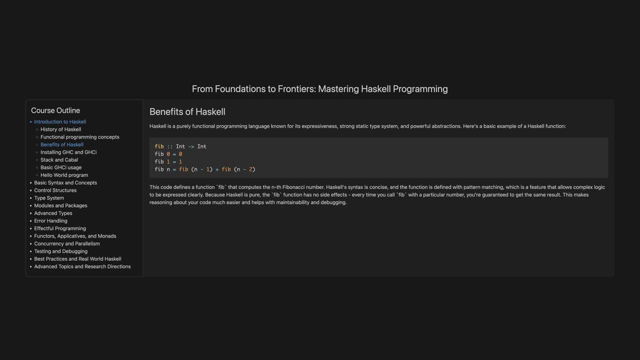 language known for its expressiveness, strong static type system and powerful abstractions. Here's a basic example of a Haskell function. This code defines a function, fib, that computes the nth Fibonacci number. Haskell's syntax is concise and the function is defined with pattern matching, which is: 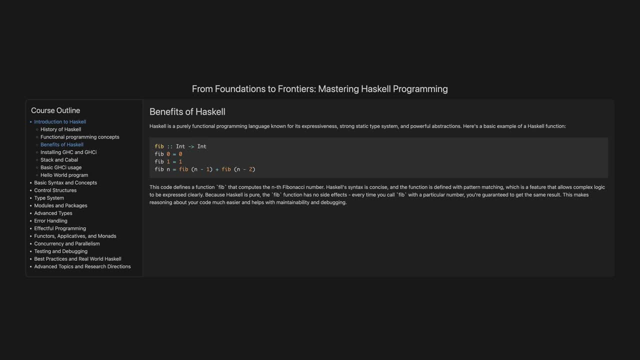 a feature that allows complex logic to be expressed clearly. Because Haskell is pure, the fib function has no side effects. Every time you call fib with a particular number, you're guaranteed to get the same result. This makes reasoning about your code much easier and helps with maintainability. and 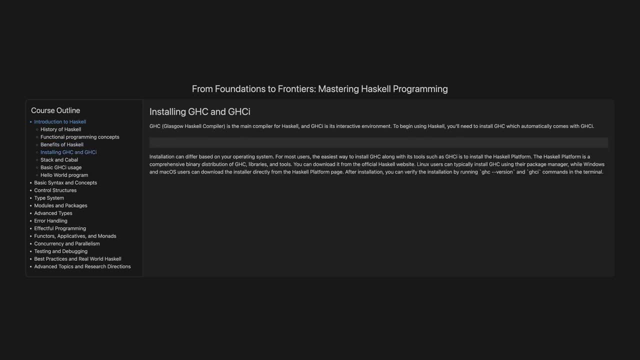 debugging: Installing GHC and GHCI. GHC is the main compiler for Haskell and GHCI is its interactive environment. To begin using Haskell, you'll need to install GHC, which automatically comes with GHCI. Installation can differ based on your operating system. 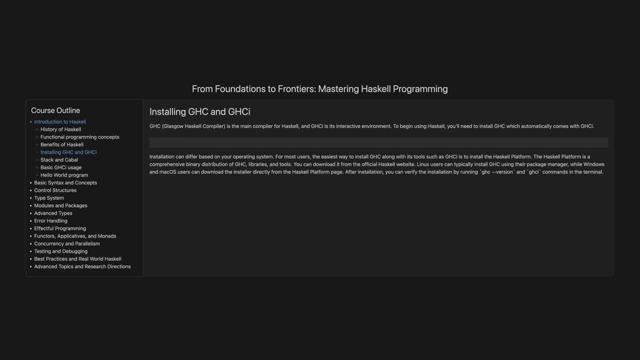 For most users, the easiest way to install GHC along with its tools is to install the Haskell platform. The Haskell platform is a comprehensive binary distribution of GHC libraries and tools. You can download it from the official Haskell website. Linux users can typically install GHC using their package manager, while Windows and Mac 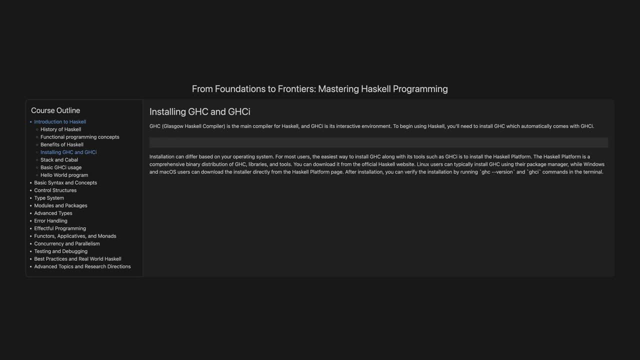 OS users can download the installer directly from the Haskell platform page. After installation: you can verify the installation by running ghc version and ghci commands in the terminal Installing Haskell Stack and Cabal. Stack and Cabal are both tools for Haskell project management. 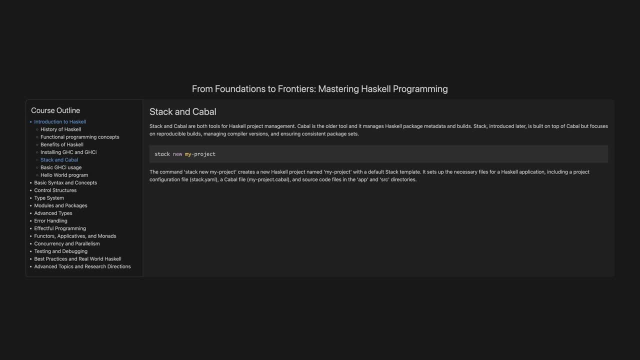 Cabal is the older tool and it manages Haskell package metadata and builds. Stack introduced later is built on top of Cabal but focuses on reproducible builds, managing compiler versions and ensuring consistent package sets. The command stack new myproject creates a new Haskell project named myproject, with 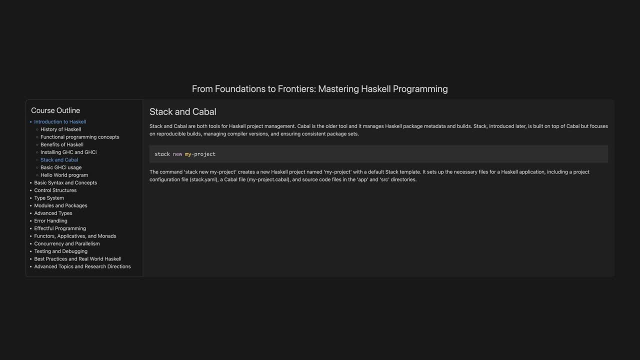 a default stack template. It sets up the necessary files for a Haskell application, including a project configuration file, stackyaml, a cabal file- myprojectcabal- and source code files in the app and src directories. Basic GHCI Usage: GHCI is the interactive environment for GHC, the Glasgow Haskell compiler. 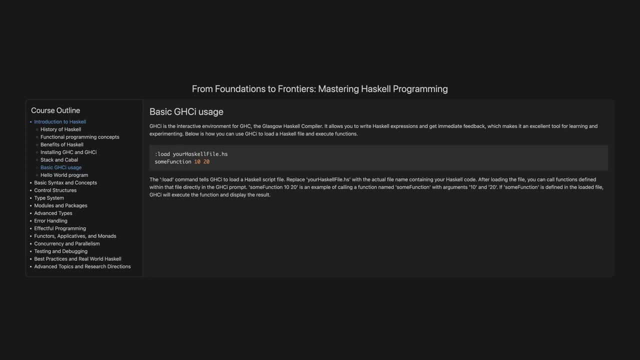 It allows you to write Haskell expressions and get immediate feedback, which makes it an excellent tool for learning and experimenting. Below is how you can use GHCI to load a Haskell file. You can download the Haskell file from the Haskell library. You can download the Haskell file from the Haskell library. 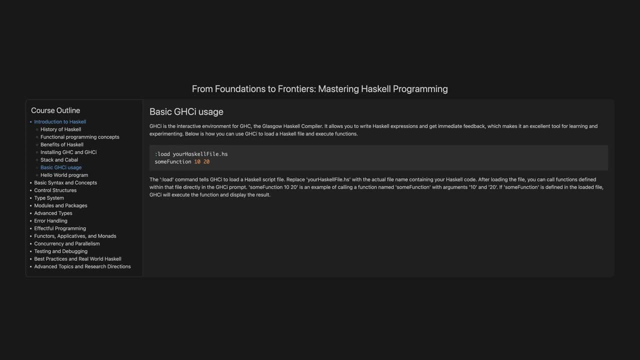 You can handle the Haskell file and execute functions. The load command tells GHCI to load a Haskell script file. Replace your Haskell filehs with the actual file name containing your Haskell code. After loading the file, you can call functions defined within that file directly in the GHCI. 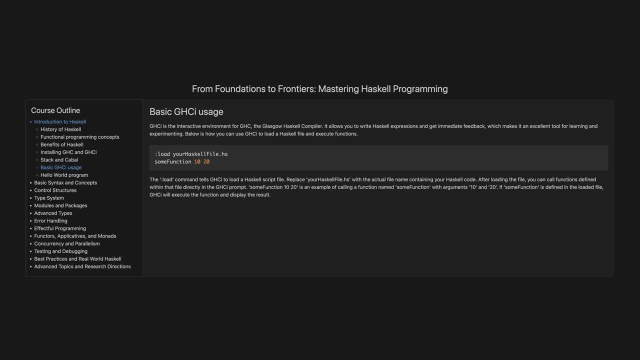 prompt Some function. 10- 20 is an example of calling a function named some function with arguments 10 and 20.. If some function- 10,, 20 or 10.20- is defined in the loaded file, GHCI will execute the. 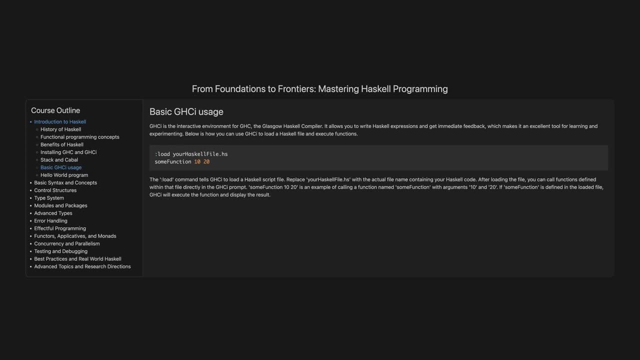 HCI will execute the function and display the result. Hello World program. The Hello World program is often the first step in learning a new programming language. It's a simple program that outputs the phrase Hello World on the screen In Haskell. we'll write this program showcasing the structure and syntax of a basic Haskell. 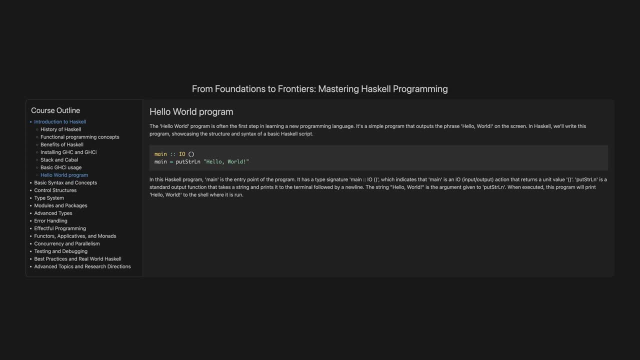 script. In this Haskell program, main is the entry point of the program. It has a type signature, main I O, which indicates that main is an I O input output action that returns a unit value. Put star L- N is a standard output function that takes a string and prints it to the terminal. 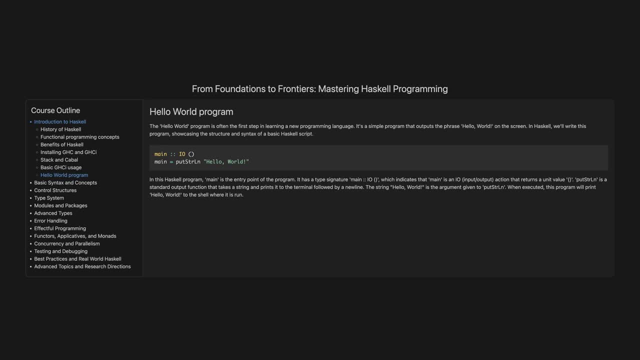 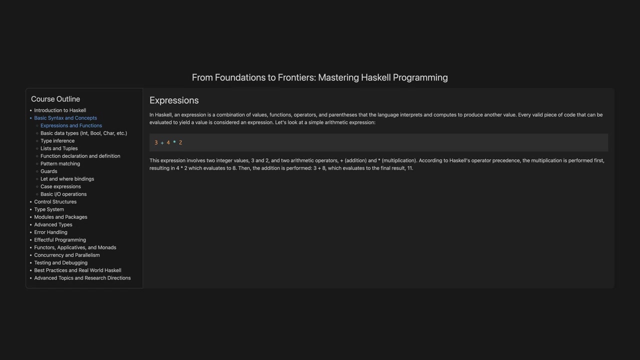 followed by a new line. The string Hello World is the argument given to put star L- N. When executed, this program will print Hello World to the shell where it is run. Expressions and functions. In Haskell, an expression is a combination of values, functions, operators and parentheses. 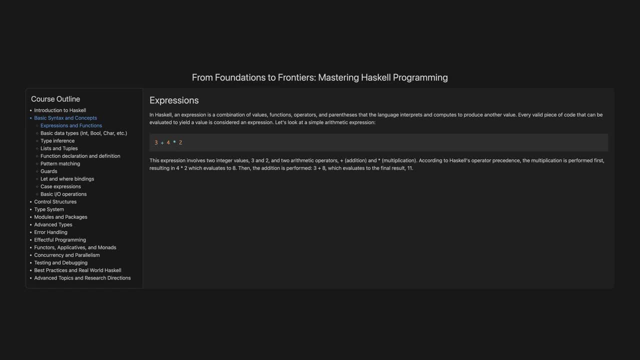 that the language interprets and computes to produce another value. Every valid piece of code that can be evaluated to yield a value is considered an expression. Let's look at a simple arithmetic expression. This expression involves two integer values, 3 and 2, and two arithmetic operators plus. 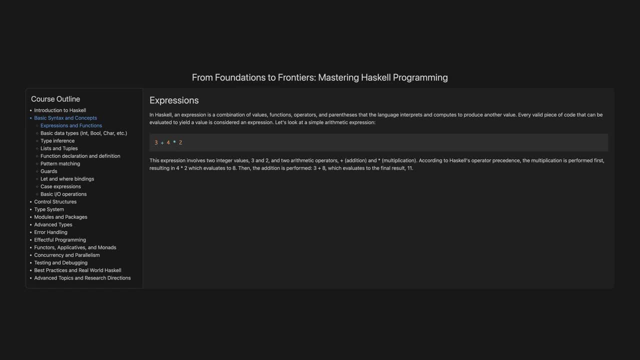 addition and store multiplication. First an integer is performed, 3 plus 8, which evaluates to the final result. 11. Basic data types: int, bool, char, etc. In Haskell, basic data types include int for integers, bool for Boolean values and char. 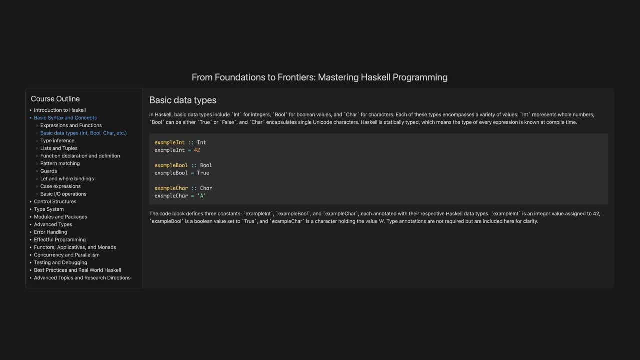 for characters. Each of these types encompasses a variety of values: Int represents whole numbers, Bool can be either true or false And char encapsulates single Unicode characters. Haskell is statically typed, which means the type of every expression is known at compile time. 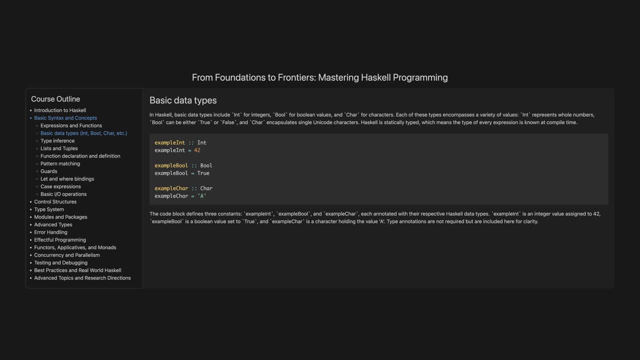 The code block defines three constants: example int, example bool and example char, each annotated with their respective Haskell data types. Example int is an integer value assigned to 42.. Example bool is a Boolean value set to true And example char is a character holding the value a. 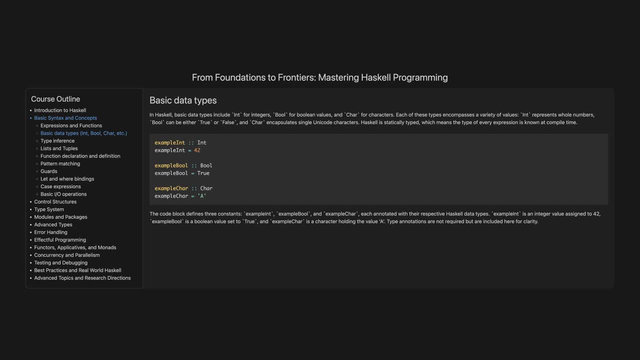 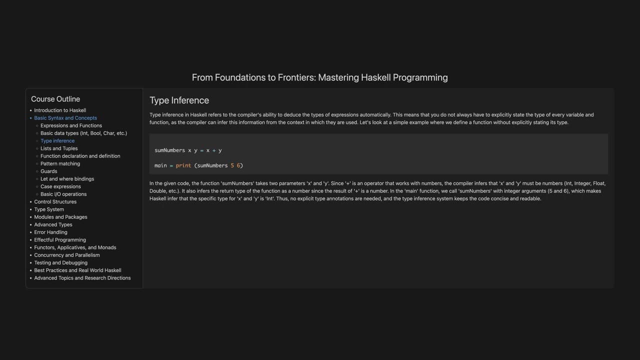 Type annotations are not required, but are included here. Type inference in Haskell refers to the compiler's ability to deduce the types of expressions automatically. This means that you do not always have to explicitly state the type of every variable and function, as the compiler can infer this information from the context in which they. 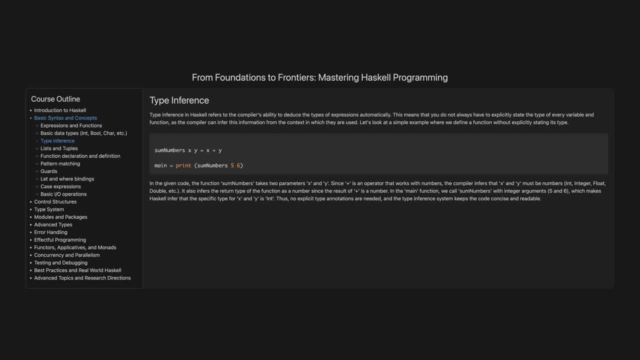 are used. Let's look at a simple example where we define a function without explicitly stating its type. In the given code, the function sumNumbers takes two parameters: x and y. Since plus is an operator that works with numbers, the compiler infers that x and y. 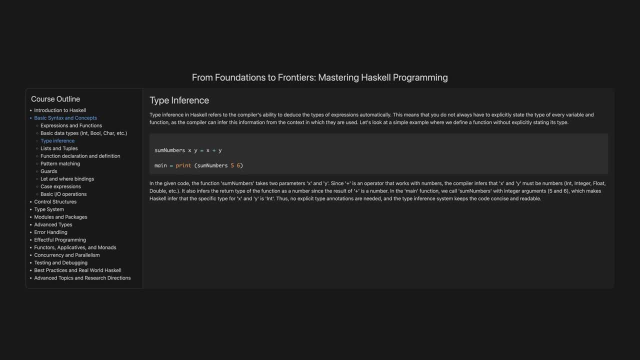 must be numbers: int, integer, float, double, etc. It also infers the return type of the function as a number, since the result of plus is a number. In the main function we call sumNumbers, with integer arguments 5 and 6, which makes Haskell. 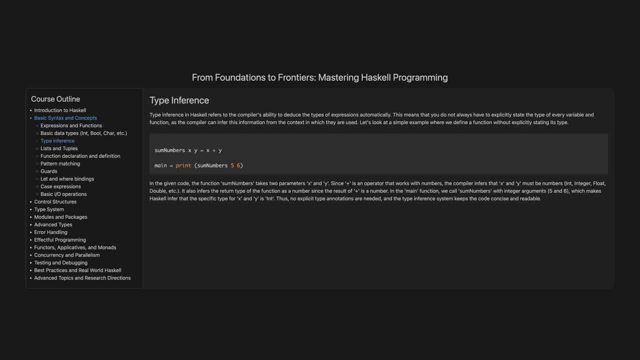 infer that the specific type for x and y is int. Thus, no explicit type annotations are needed And the type inference system keeps the code concise and readable. Lists and Tuples. In Haskell, a list is a collection of elements of the same type. 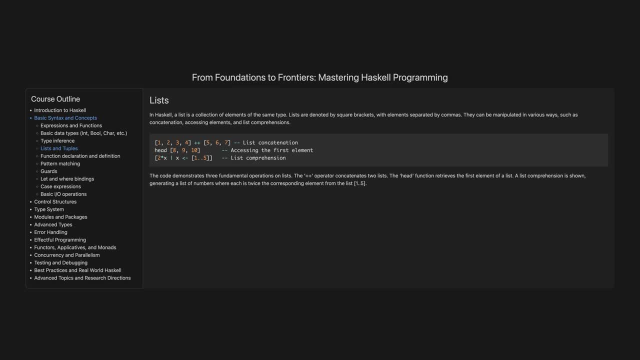 Lists are denoted by square brackets, with elements separated by commas. They can be manipulated in various ways, such as concatenation, accessing elements and list comprehensions. The code demonstrates three fundamental operations on lists: 1. Concatenation, 2.. 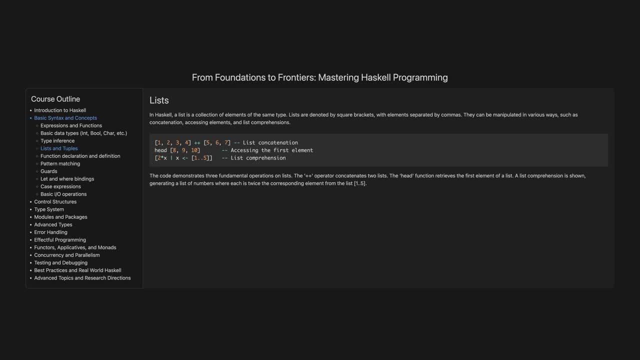 List Comprehension. The plus plus operator concatenates two lists. The head function retrieves the first element of a list. A list comprehension is shown, generating a list of numbers where each is twice the corresponding element from the list 1, 5.. 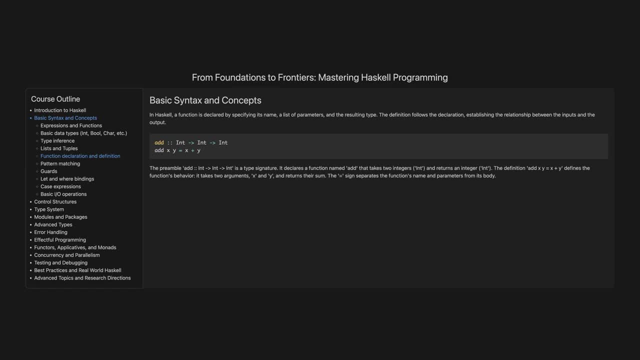 Function Declaration and Definition. In Haskell, a function is declared by specifying its name, a list of parameters and the resulting type. The definition follows the declaration: 1. Add to Int- Int. Int. The definition. Add xy equals x plus y defines the function's behaviour. 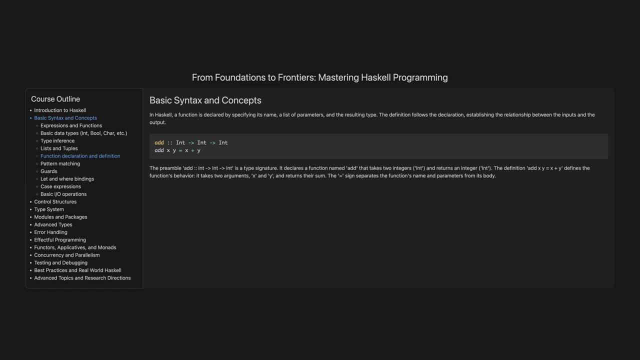 It takes two arguments, x and y, and returns their sum. The equals sign separates the function's name and parameters from its body. 2. Pattern Matching 3. in Haskell allows you to check a value against a pattern. It's a more powerful version of a. 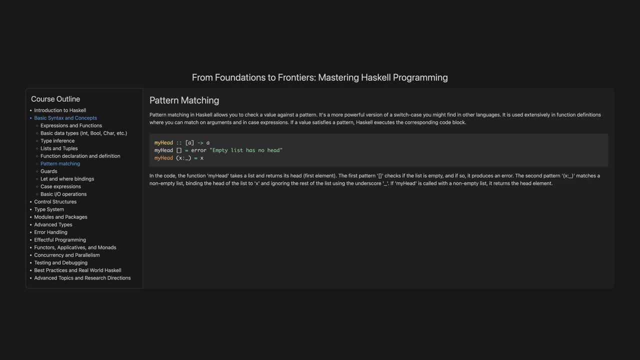 switch case you might find in other languages. It is used extensively in function definitions where you can match on arguments and in case expressions. If a value satisfies a pattern, Haskell executes the corresponding code block In the code. the function myHead takes a list. 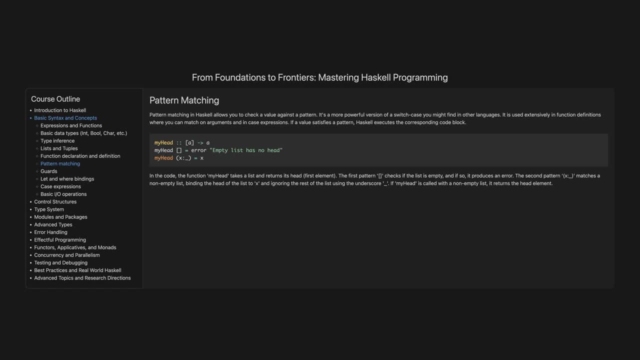 and returns its head first element. The first pattern checks if the list is empty and if so, it produces an error. The second pattern, xScore, matches a non-empty list, binding the head of the list to x and ignoring the rest of the list using the underscore 4.. 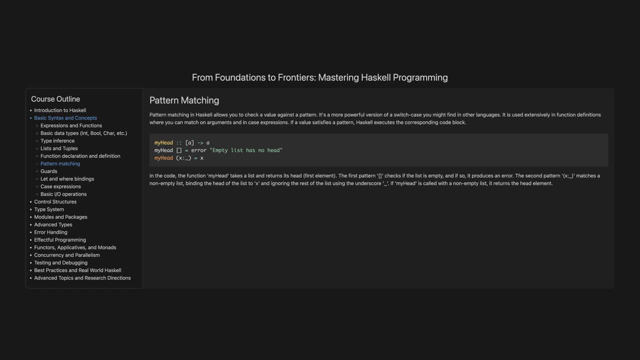 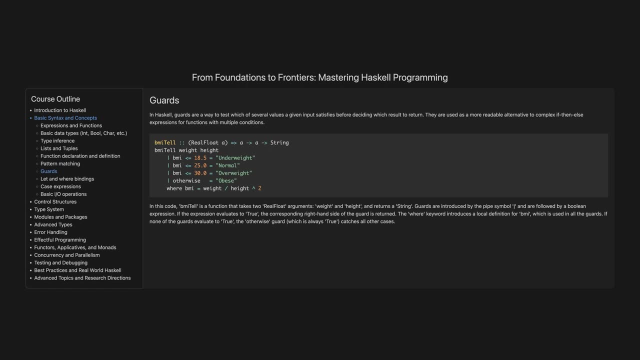 If myHead is called with a non-empty list, it returns the head element Guards. In Haskell, guards are a way to test which of several values a given input satisfies before deciding which result to return. They are used as a more readable alternative to 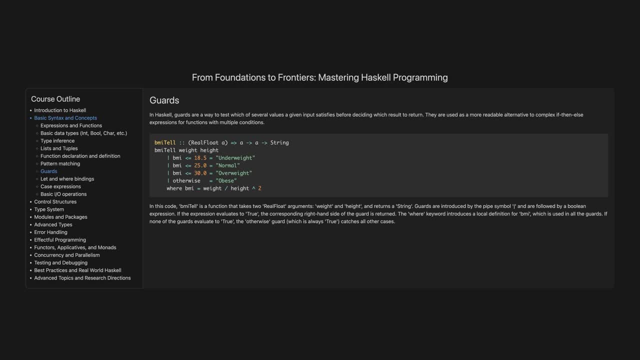 conflict. Guards are complex if-then-else expressions for functions with multiple conditions. In this code, BMI tell is a function that takes two real float arguments- weight and height- and returns a string. Guards are introduced by the pipe symbol ls and are followed by a Boolean expression If the expression evaluates to true. 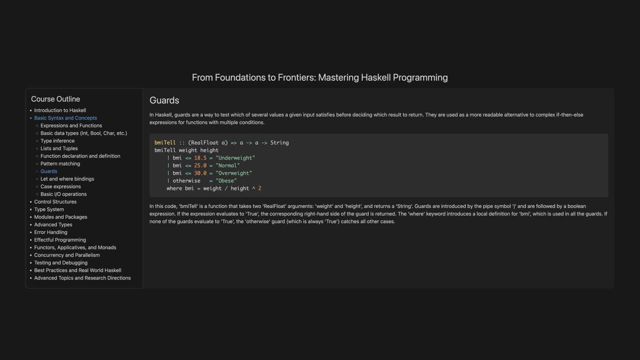 the corresponding right-hand side of the guard is returned. The where keyword introduces a local definition for BMI which is used in all the guards. If none of the guards are used, wanted to evaluate that our mention into truth. a wouldサ08 causes it to violate collection. 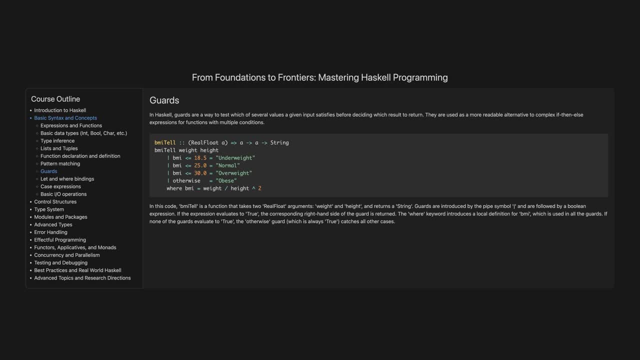 of data undertaken during the VCF perfection process. Allguards evaluate to true the otherwise guard, which is always true, catching all other cases. Let and where bindings. In Haskell, let bindings allow us to define local variables within an expression. The general syntax is: let bindings in expression. 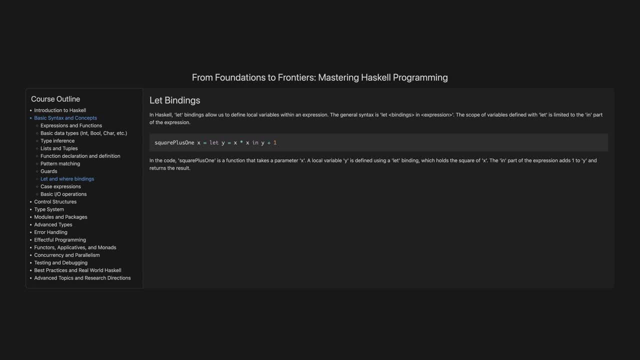 The scope of variables defined with let is limited to the in part of the expression In the code. square plus one is a function that takes a parameter x. a local variable, y, is defined using a let binding which holds the square of x, the in part of the expression. 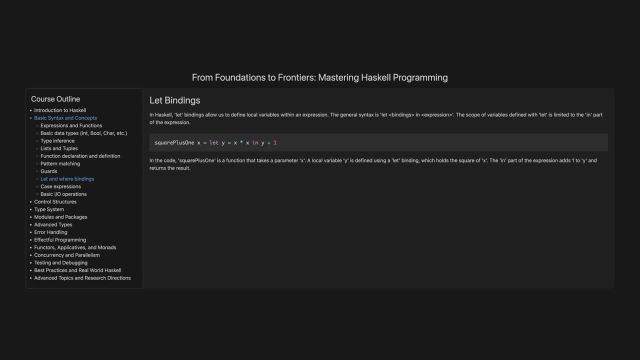 adds 1 to y and returns the result. case expressions. in haskell, the case expression allows you to evaluate an expression and branch the code depending on the value of the evaluation. this is similar to the switch case statement in imperative languages. it's particularly useful for pattern matching against complex data types, allowing for more readable and expressive code. 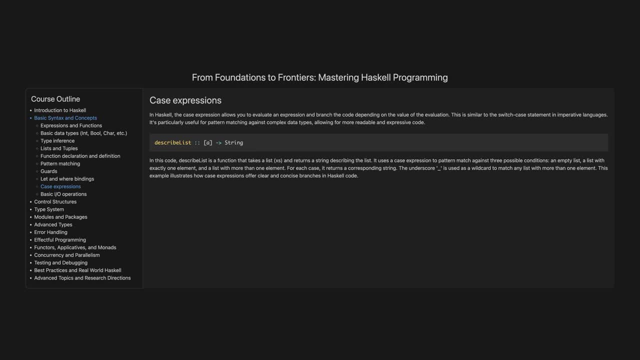 in this code. describe list is a function that takes a list xs and returns a string describing the list. it uses a case expression to pattern match against three possible conditions: an empty list, a list with exactly one element and a list with more than one element for each case. 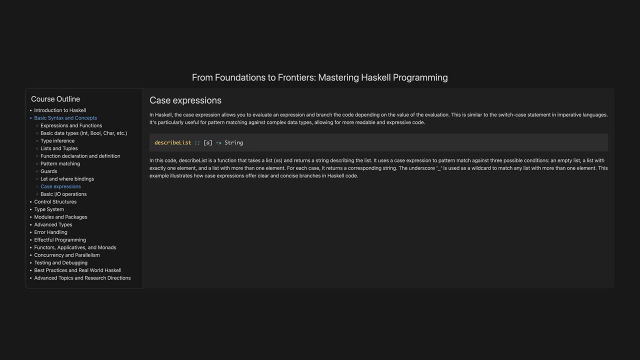 it returns a corresponding string. the underscore score is used as a wild card to match any list with more than one element. this example illustrates how case expressions offer clear and concise branches in haskell code basic i o operations. in haskell i o, operations are: 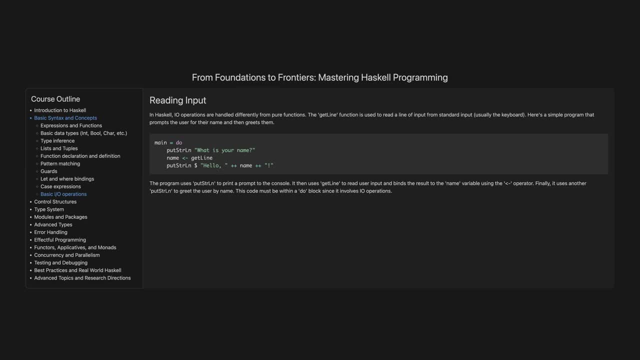 handled differently from pure functions. the get line function is used to read a line of input from standard input, usually the keyboard. here's a simple program that prompts the user for their name and then greets them. the program uses put star ln to print a prompt to the console. 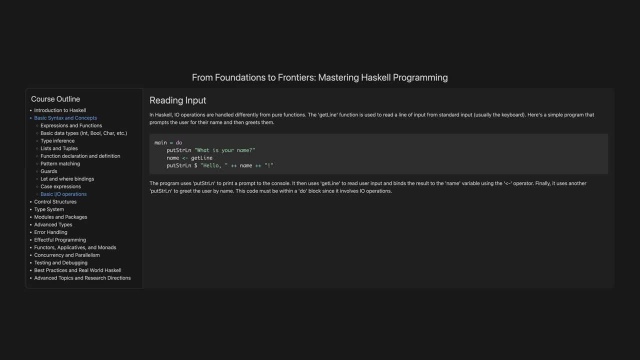 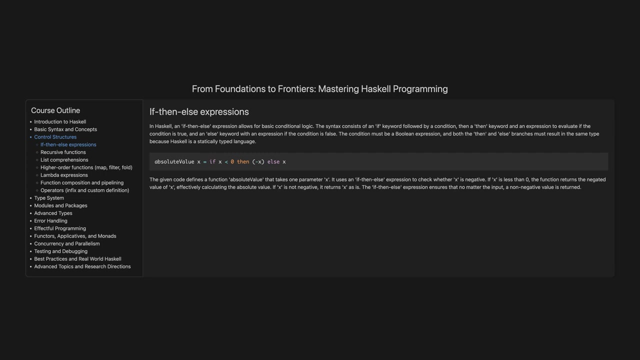 it then uses get line to read user input and binds the result to the name variable using the snads operator. finally, it uses another put star n to greet the user by name. this code must be within a do block, since it involves io operations. if then else expressions in haskell, an if then else expression allows for basic conditional. 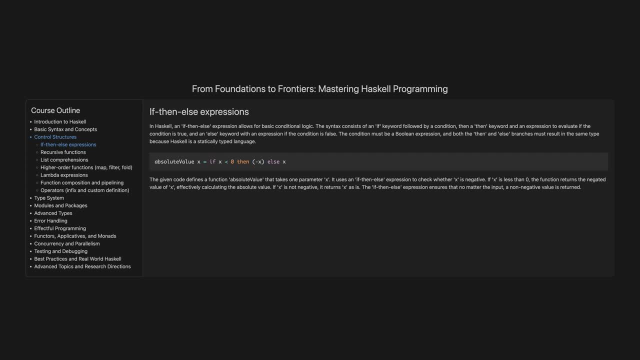 logic. the syntax consists of an if keyword followed by a condition, then a then else keyword and an expression to evaluate if the condition is true, and an else keyword with an expression if the condition is false. the condition must be a boolean expression and both the then and 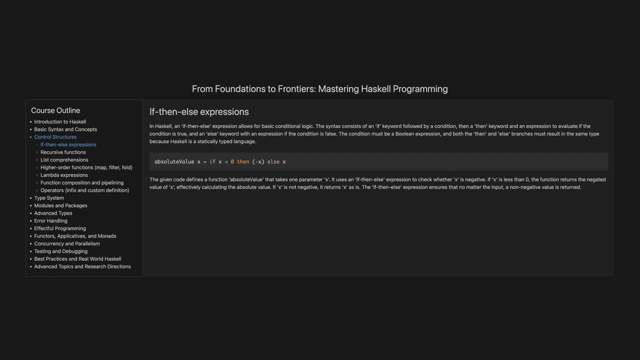 else branches must result in the same type, because haskell is a statically typed language. the given code defines a function, absolute value- that takes one parameter, x. it uses an if then else expression to check whether x is negative. if x is less than zero, the function returns the negate. 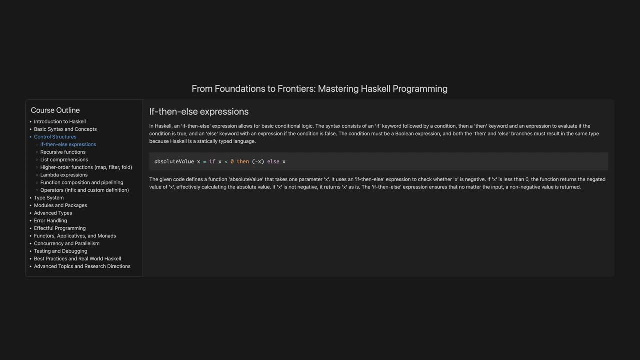 value of x, effectively calculating the absolute value. if x is not negative, it returns x, as is the if, then else expression ensures that, no matter the input, a non-negative value is returned. recursive functions: in haskell, recursion is a fundamental concept where a function calls itself to solve a problem. a well-defined recursive function. 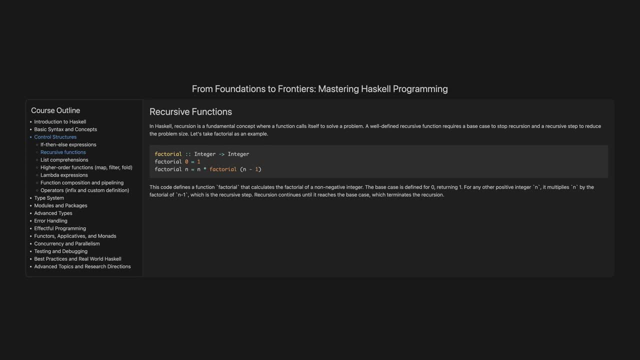 requires a base case to stop recursion and a recursive step to reduce the problem state size. let's take factorial as an example. this code defines a function factorial that calculates the factorial of a non-negative integer. the base case is defined for 0, returning 1.. for any other: 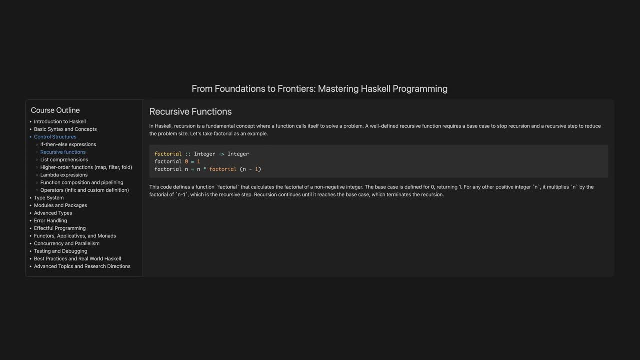 positive integer n. it multiplies n by the factorial of n minus 1, which is the recursive step. recursion continues until it reaches the base case, which terminates the recursion list. comprehensions- list comprehensions in haskell are a concise way to create lists based on existing lists. they are similar to the set. 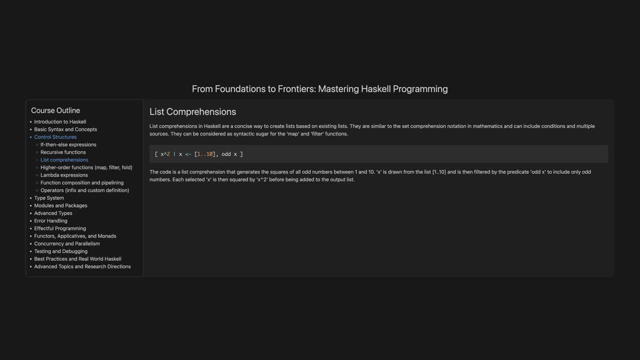 comprehension notation in mathematics and can include conditions and multiple sources. they can be considered as syntactic sugar for the map and filter functions. the code is a list comprehension that generates the squares of all odd numbers between 1 and 10.. x is drawn from the list 1- 10 and is then filtered by the predicate odd x to include only odd numbers. 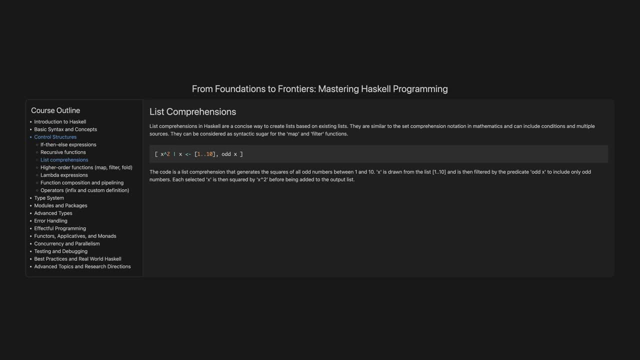 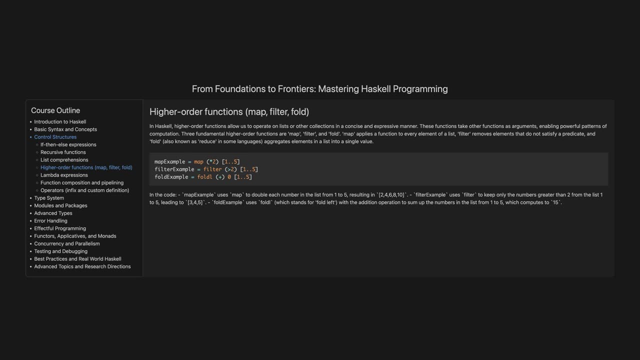 x is then squared by x squared before being added to the output list. higher order functions- map filter fold in haskell. higher order functions allow us to operate on lists or other collections in a concise and expressive manner. these functions take other functions as arguments, enabling powerful patterns. 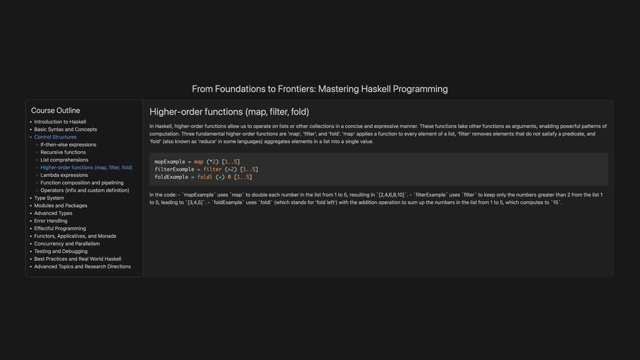 of computation. three fundamental higher order functions are map, filter and fold. map applies a function to every element of a list. filter removes elements that do not satisfy a predicate, and fold, also known as reduce in some languages, aggregates elements in a list into a single value in the code. 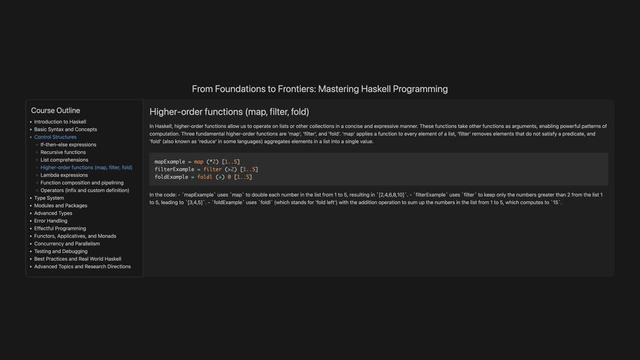 map example. uses map to double each number in the list from 1 to 5, resulting in 2, 4, 6, 8, 10. filter example: uses filter to keep only the numbers greater than 2 from the list 1 to 5, leading to 3, 4, 5.. 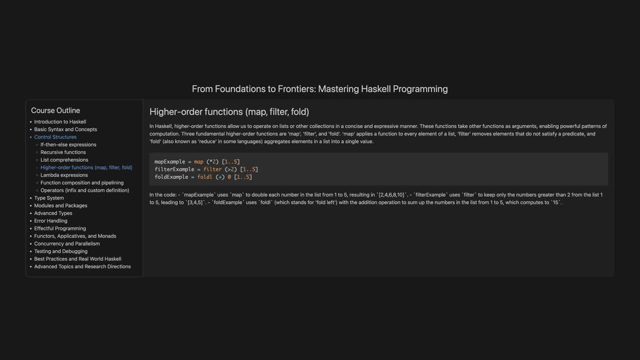 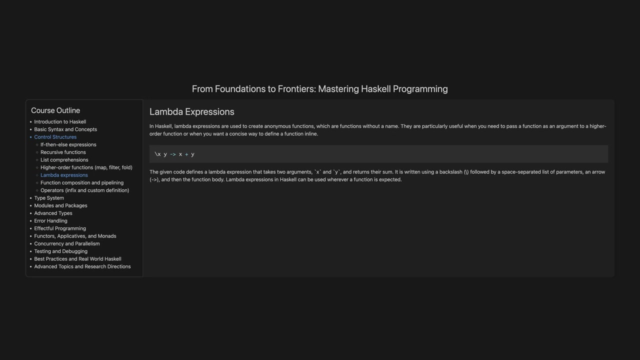 fold. example uses foldle, which stands for fold left, with the addition operation to sum up the numbers in the list from 1 to 5, which computes to 15.. lambda expressions: in haskell, lambda expressions are used to create anonymous functions, which are functions without a name. they are particularly useful when you need to pass a. 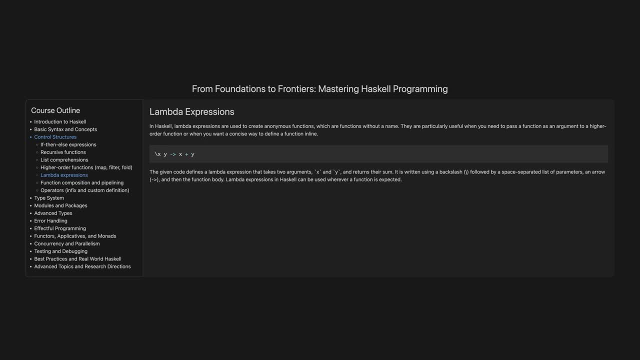 function as an argument to a higher order function or when you want a concise way to define a function in line. the given code defines a lambda expression that takes two arguments, x and y, and returns their sum. it is written using a backslash, followed by a space separated. list of parameters: an arrow. 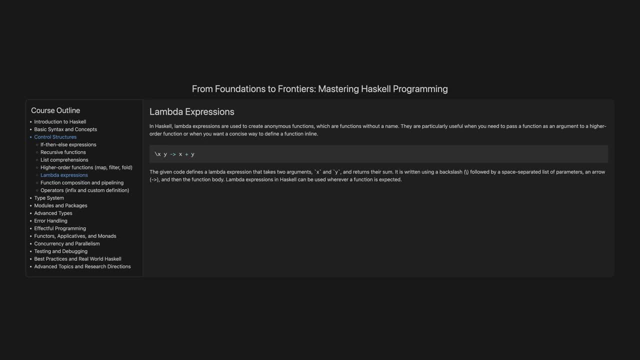 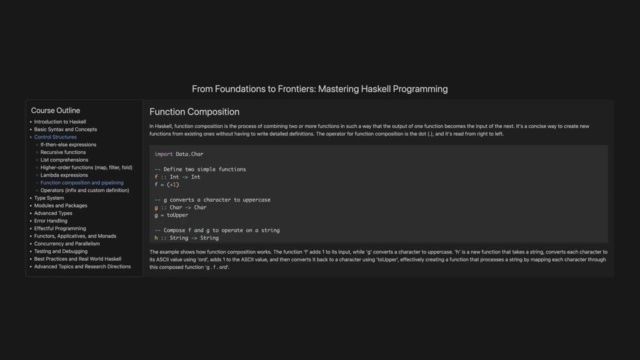 and then the function body. lambda expressions in haskell can be used wherever a function is expected. function composition and pipelining in haskell function composition is the process of combining two or more functions in such a way that the output of one function becomes the. 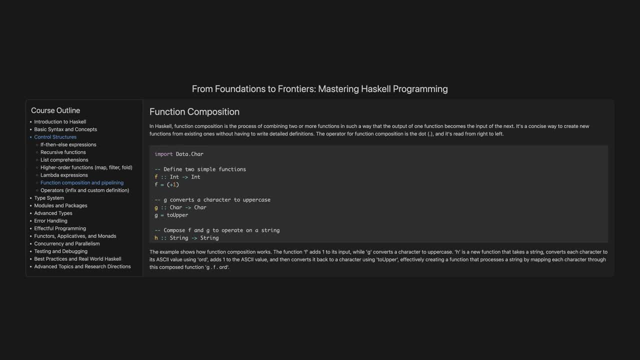 input of the next. it's a concise way to create new functions from existing ones without having to write detailed definitions. the operator for function composition is the dot, and it's read from right to left. the example shows how function composition works. the function f adds one to its input, while g converts a character to uppercase. h is a new function that takes a. 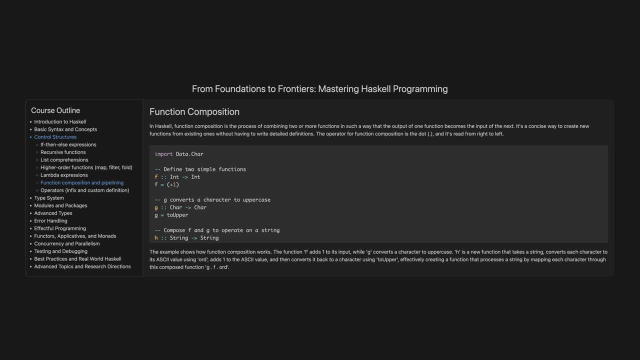 string and converts a character to uppercase. the function f is a new function that takes a string, converts each character to its ascii value using odd, adds one to the ascii value and then converts it back to a character using two upper, effectively creating a function that processes a string by 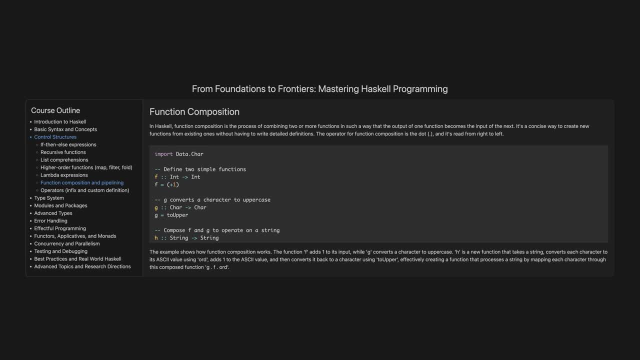 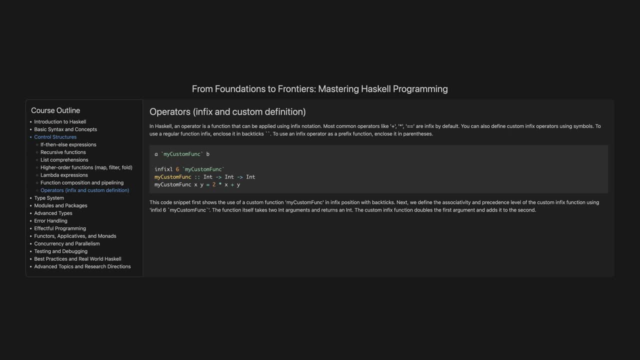 mapping each character through this composed posed: function g, f, odd operators, infix and custom definition. in haskell, an operator is a function that can be applied using infix notation- most common operators like plus tool, equals, equals or infix by default. you can also define custom infix operators using symbols to use a regular 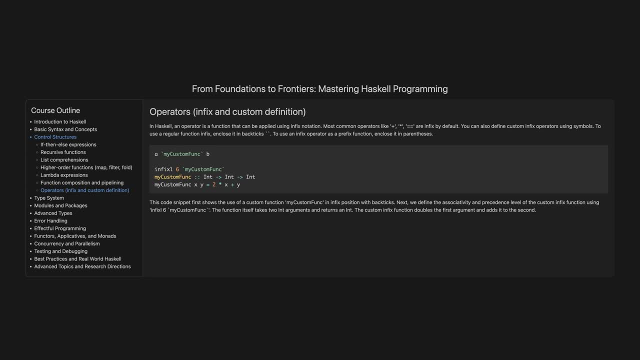 function infix. enclose it in backticks to use an infix operator as a prefix function. enclose it in parentheses. this code snippet first shows the use of a custom function- my custom funk- in infix position with backticks. next we define the associativity and precedence level of the 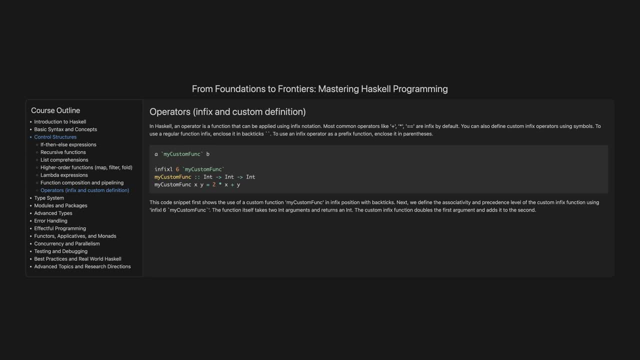 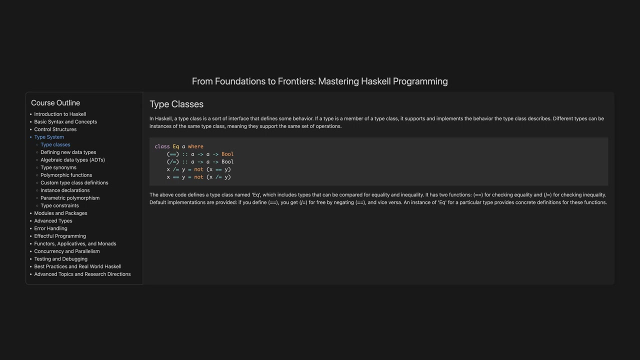 custom infix function using infixel6, my custom funk. the function itself takes two int arguments: int. the custom infix function doubles the first argument and adds it to the second. type classes. in haskell, a type class is a sort of interface that defines some behavior. if a type is a member of a type class, it supports and implements the behavior. the: 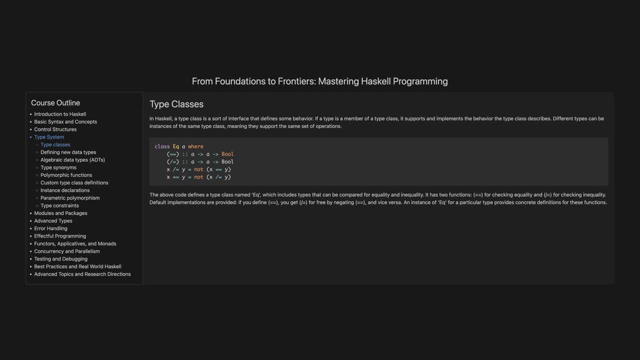 type class describes different types can be instances of the same type class, meaning they support the same set of operations. the above code defines a type class named eq, which includes types that can be compared for equality and inequality. it has two functions: call 6 for checking equality. 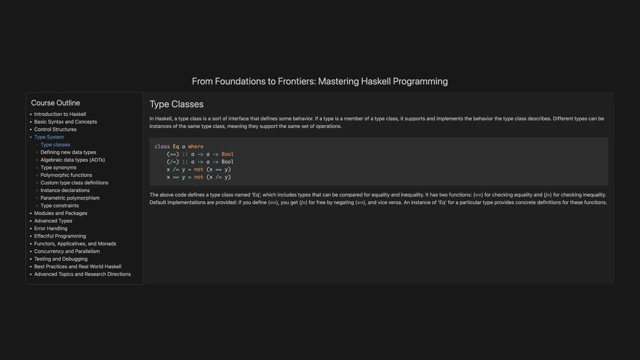 and slash equals for checking inequality. default implementations are provided. if you define corporate, you get three for free by negating quick and vice versa. an instance of eq for a particular type provides concrete definitions for these functions. defining new data types. in haskell you can define new data types using the data keyword. 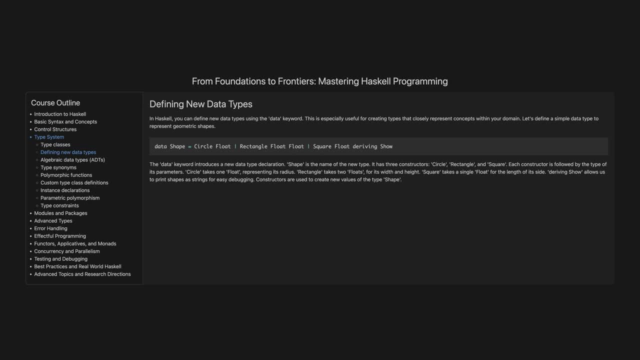 this is especially useful for creating types that closely represent concepts within your domain. let's define a simple data type to represent geometric shapes. the data keyword introduces a new data type declaration. shape is the name of the new type. it has three constructors: circle, rectangle and square. each constructor is followed by the type of its parameters. 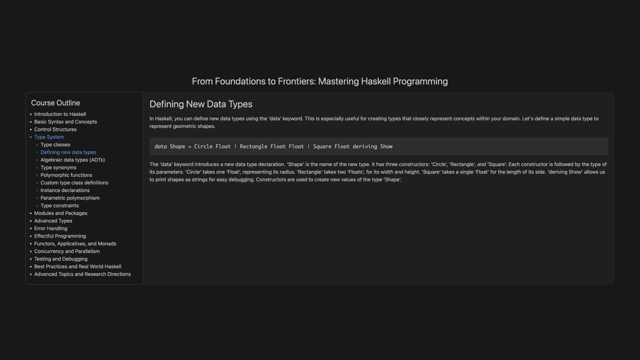 circle takes one float representing its radius. rectangle takes two floats for its width and height. square takes a single float for the length of its side. deriving show allows us to print shapes as strings for easy debugging. constructors are used to create new values of the type shape. algebraic data types- adts. algebraic data types are a way to define custom data types in haskell. 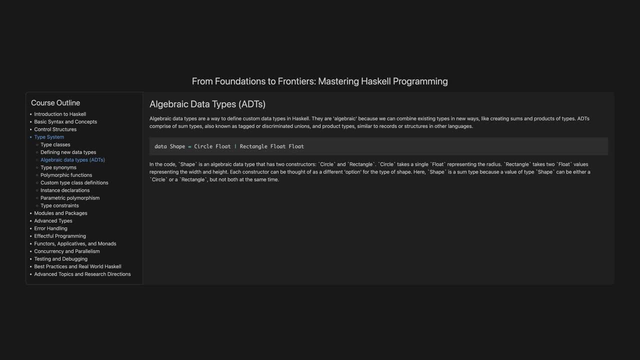 they are algebraic because we can combine existing types in new ways, like creating sums and products of types. adts comprise of some types also known as tagged or discriminated unions, and product types similar to records or structures in other languages. in the code shape is an algebraic data type that has two constructors: circle and 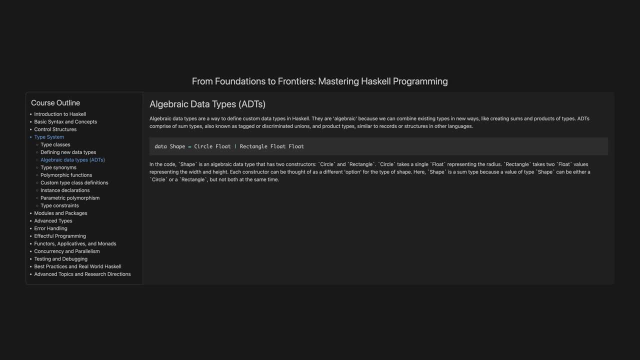 rectangle circle takes a single float representing the radius. rectangle takes two float values representing the width and height. each constructor can be thought of as a different option for the type of shape. here shape is a sum type. as a value of type, shape can be used to define a type shape. 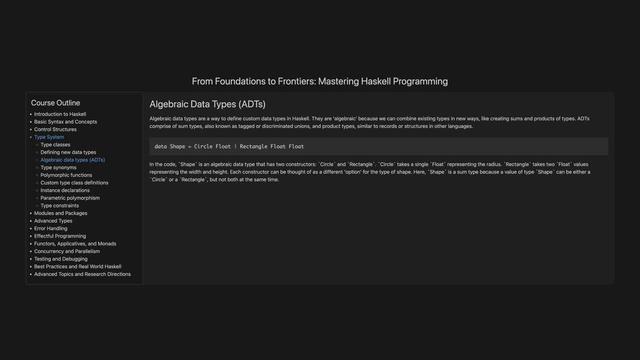 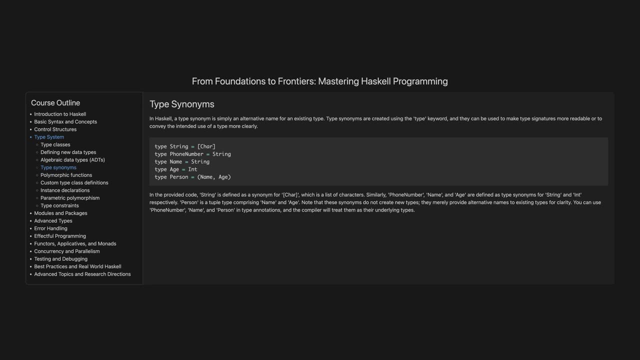 and a type which is a combination of a type shape and a type shape. type synonyms. in haskell, a type synonym is simply an alternative name for an existing type. type synonyms are created using the type keyword and they can be used to make type signatures more. 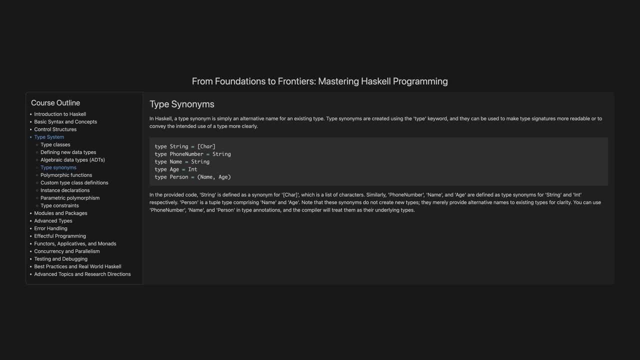 readable or to convey the intended use of a type more clearly. in the provided code, string is defined as a synonym for char, which is a list of characters. similarly, phone number, name and age are defined as type synonyms for string and int respectively. Person is a tuple type comprising name and age. Note that these synonyms do not create new types. 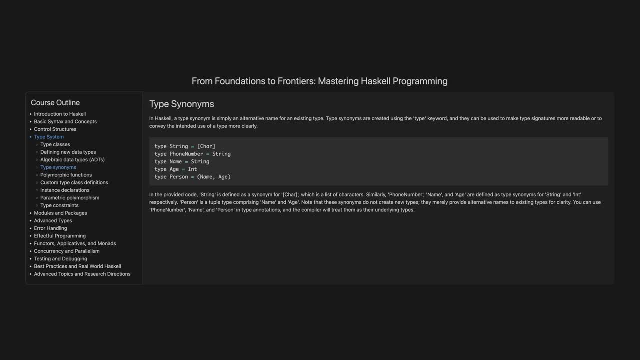 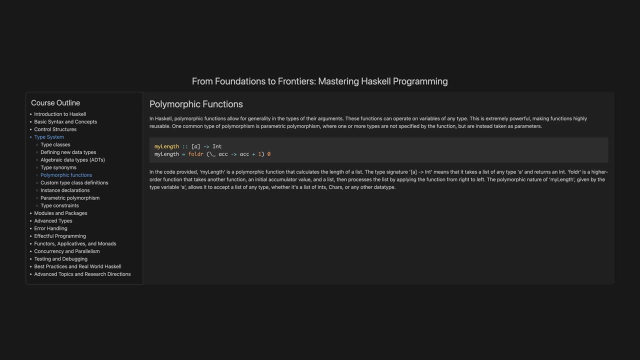 they merely provide alternative names to existing types. for clarity, You can use phone number, name and person in type annotations, and the compiler will treat them as their underlying types. Polymorphic functions In Haskell. polymorphic functions allow for generality in the types of their arguments. These functions can operate on variables of any type. 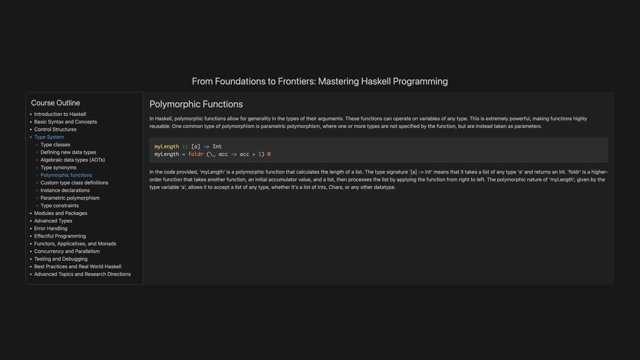 This is extremely powerful, making functions highly reusable. One common type of polymorphism is parametric polymorphism, where one or more types are not specified by the function, but are instead taken as parameters In the code provided. myLength is a polymorphism. 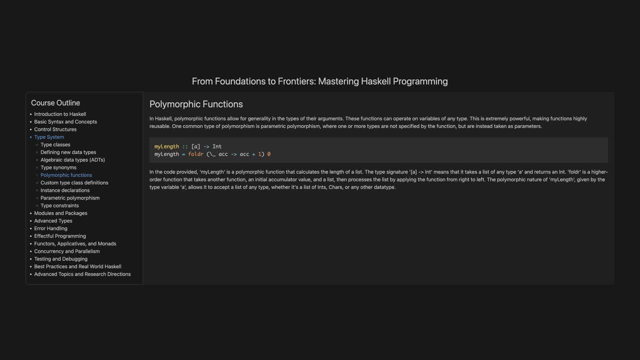 Polymorphic function that calculates the length of a list, The type signature, a int means that it takes a list of any type a and returns an int. Folder is a higher order function that takes another function, an initial accumulator value and a list, then processes the list by applying the function from right to left. 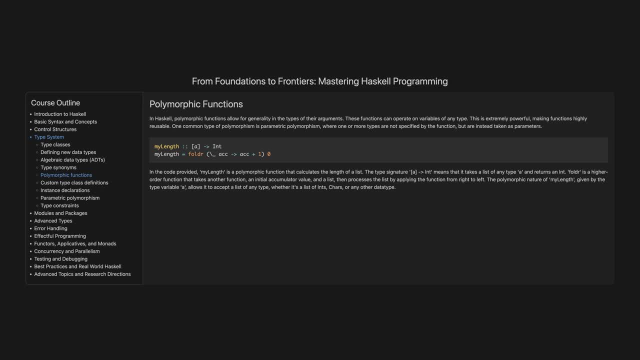 The polymorphic nature of myLength, given by the type variable a, allows it to accept a list of any type, whether it's a list of ints, chars or any other data type. The polymorphic function that calculates the length of a list of ints, chars or any other data type. 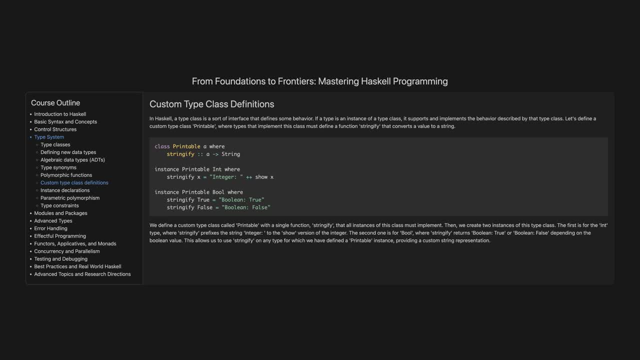 The polymorphic function that calculates the length of a list of ints, chars or any other data type. Custom type class definitions. In Haskell, a type class is a sort of interface that defines some behavior. If a type is an instance of a type class, it supports and implements the behavior described. 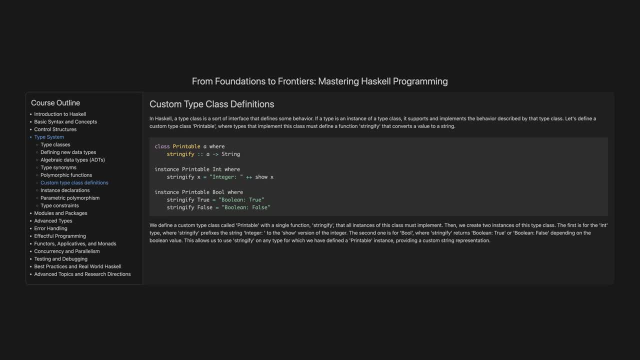 by that type class. Let's define a custom type class, printable, where types that implement this class must define a function stringify that converts a value to a string. We define a custom type class called printable, with a single function Stringify that all instances of this class must implement. 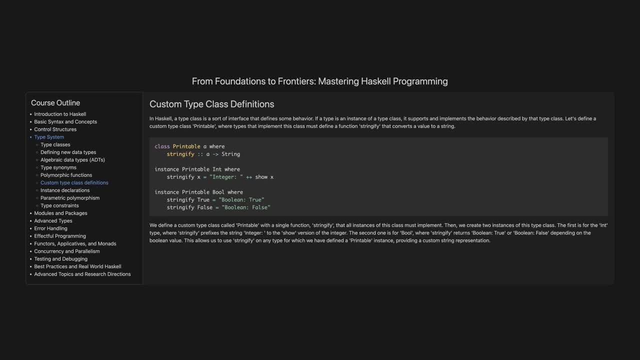 Then we create two instances of this type class. The first is for the int type, where stringify prefixes the string integer to the show version of the integer. The second one is for bool, where stringify returns boolean true or boolean false, depending on the boolean value. 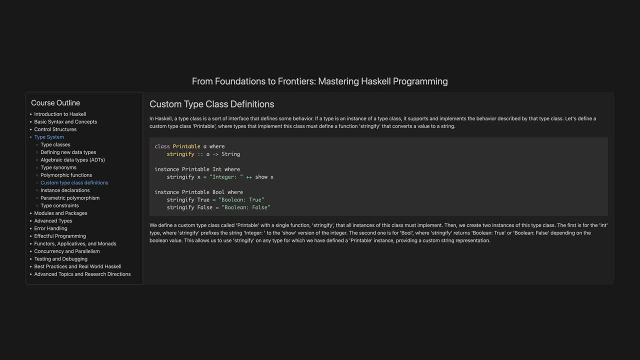 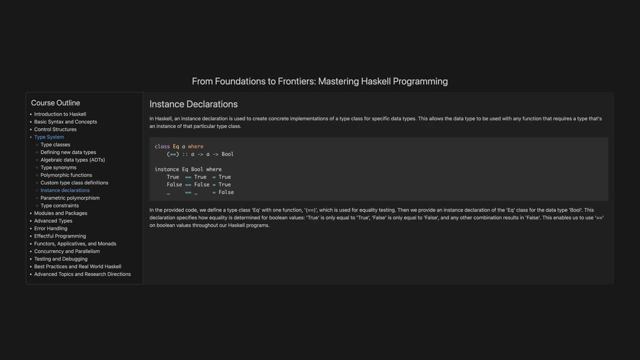 This allows us to use stringify on any type for which we have defined a printable instance providing a custom string representation. Instance declarations. In Haskell, an instance declaration is used to create concrete implementations of a type class for specific data types. This allows the data type to be used with. 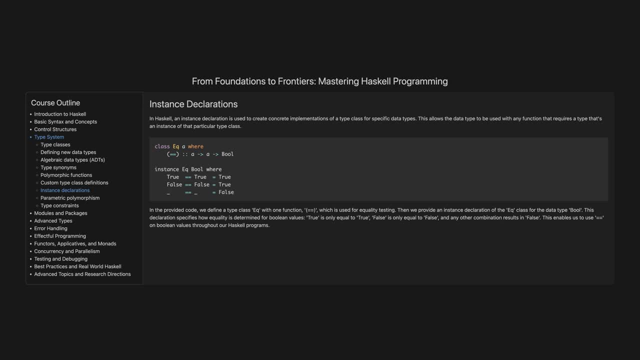 any function that requires a type. that's an instance of that particular type class. In the provided code we define a type class, eq, with one function equal, which is used for equality testing. Then we provide an instance declaration of the eq class for the data type bool. 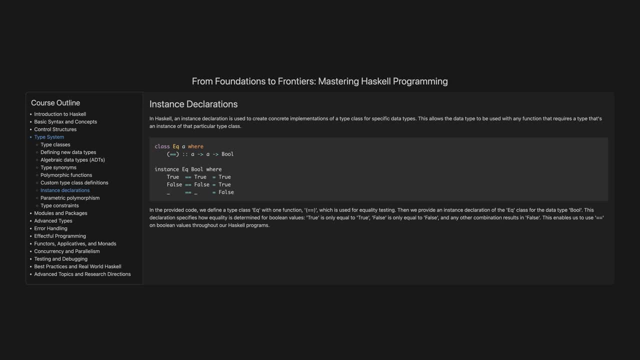 This declaration specifies how equality is determined for boolean values. True is only equal to true, false is only equal to false and any other combination results in false. This enables us to use iuxicults on boolean values throughout our Haskell programs. Parametric polymorphism. 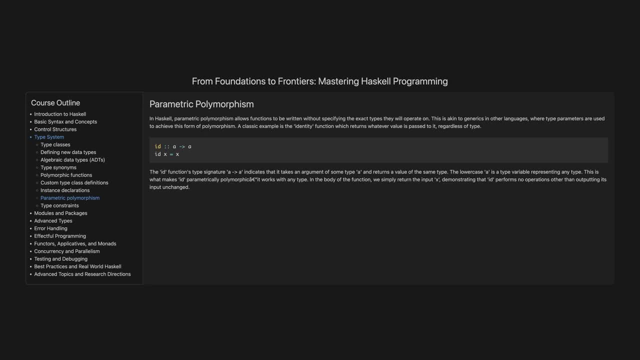 In Haskell. parametric polymorphism allows functions to be written without specifying the exact types they will operate on. This is akin to generics in other languages, where type parameters are used to achieve this form of polymorphism. A classic example is the identity function, which returns whatever value is passed to. 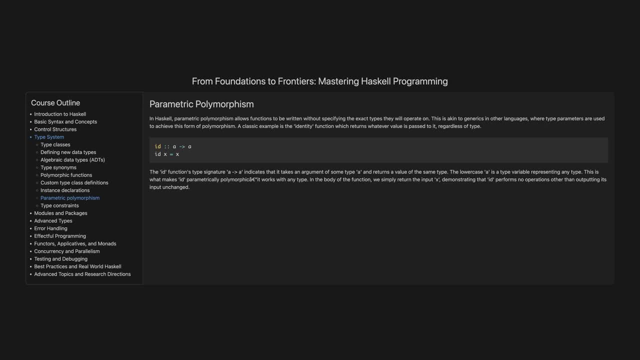 it regardless of type. The ID function's type signature a. a indicates that it takes an argument of some type a and returns a value of the same type. The lowercase a is a type variable representing any type. This is what makes ID parametrically polymorphic. 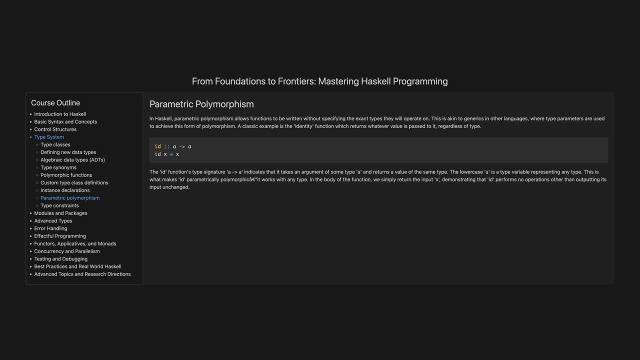 It works with any type. In the body of the function we simply return the input x, demonstrating that ID performs no operations other than outputting its input unchanged. Type constraints. In Haskell, type constraints restrict the types that can be used in a particular context. 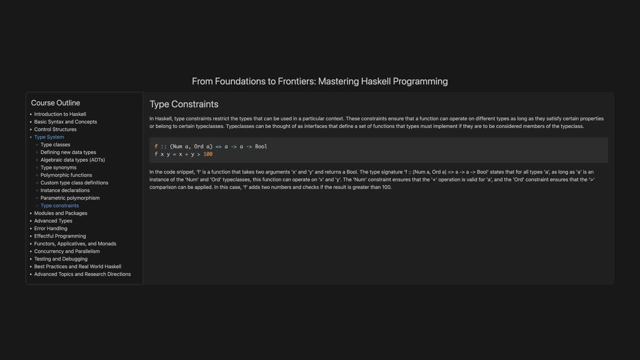 These constraints ensure that a function can operate on different types, as long as they satisfy certain properties or belong to it. This is what makes ID parametrically polymorphic. The ID function is a type variable representing any type. It works with any type. 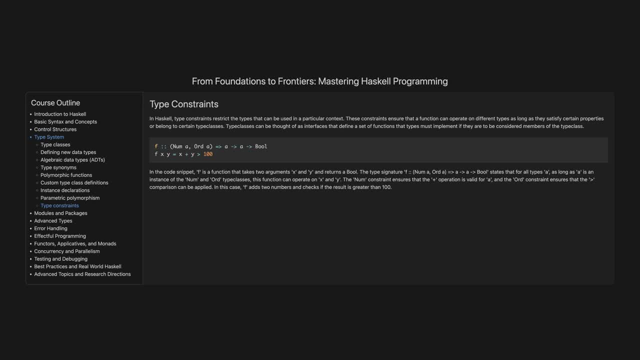 This is what makes ID parametrically polymorphic. This is what makes ID parametrically polymorphic. Type classes can be thought of as interfaces that define a set of functions that types must implement if they are to be considered members of the type class. 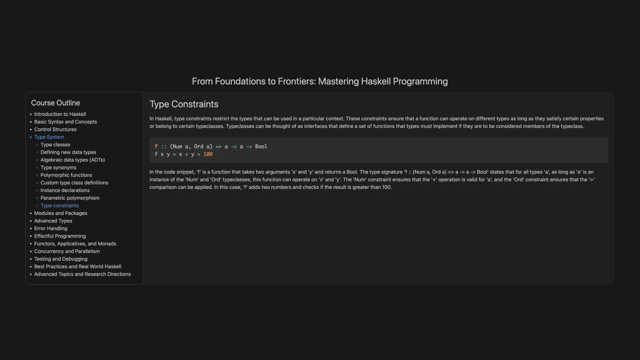 In the code snippet f is a function that takes two arguments, x and y, and returns a bool. The type signature f, numA, ordA- equals a. a mice bool states that for all types a, as long as a is an instance of the num and ord type classes, this function can operate on. 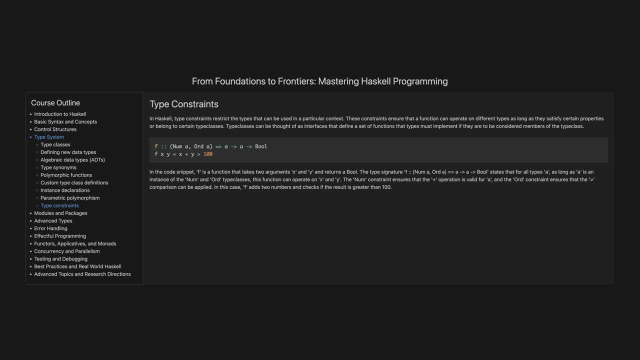 x and y. This is what makes ID parametrically polymorphic. Some constraint ensures that the plus operation is valid for a and the ord constraint ensures that the join comparison can be applied In this case. f adds two numbers and checks if the result is greater than 100. 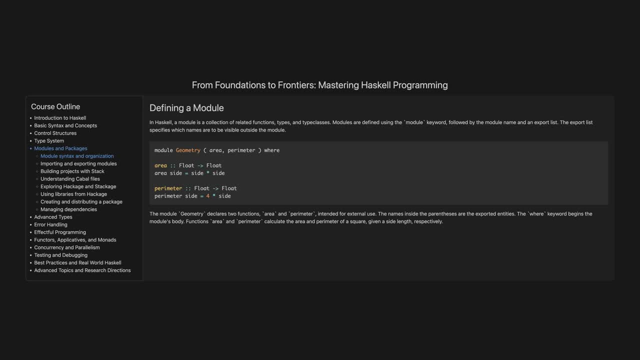 Module syntax and organization. In Haskell, a module is a collection of related functions, types and type classes. Modules are defined using the module keyword, followed by the module name and an export list. The export list specifies which names are to be visible outside the module. 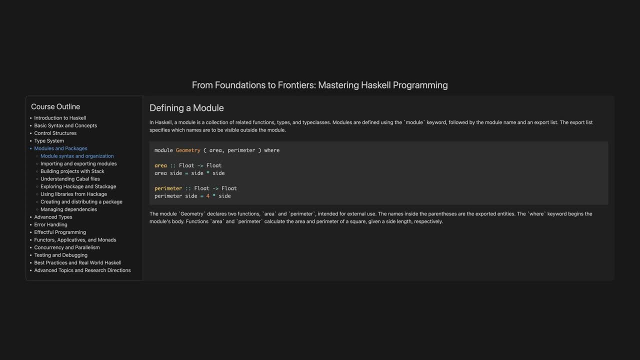 The module geometry declares two functions- area and perimeter- intended for external use. The names inside the parentheses are the exported entities. The where keyword begins the module's body Functions: area and perimeter. calculate the area and perimeter of a square given a side. 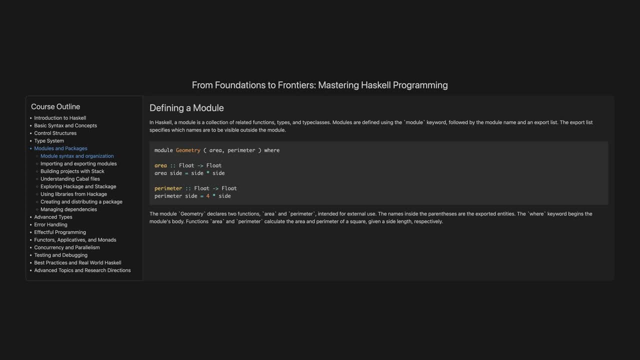 length respectively. Importing and exporting modules. Importing and exporting modules In Haskell. the name of the module is the name of the module. The name of the module is the name of the module In Haskell. modules group related functions, types and type classes. 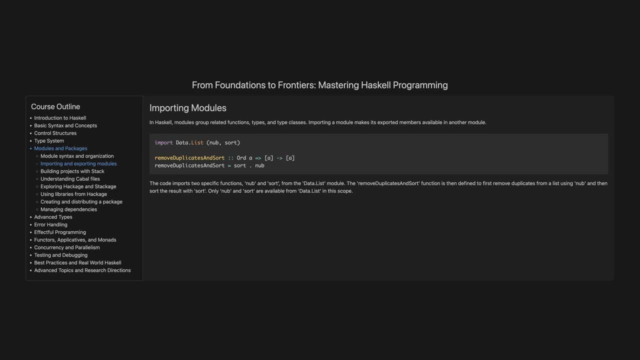 Importing a module makes its exported members available in another module. The code imports two specific functions- nub and sort- from the datalist module. The remove duplicates and sort function is then defined to first remove duplicates from a list using nub and then sort the result with sort. 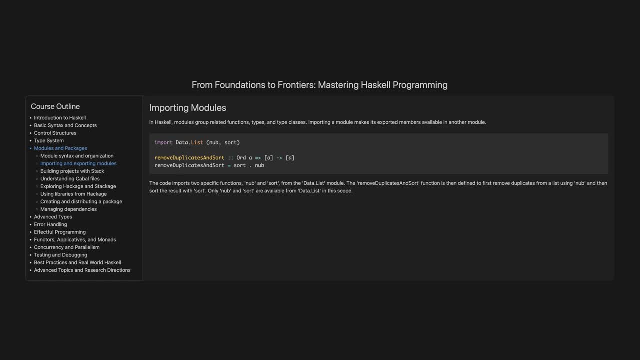 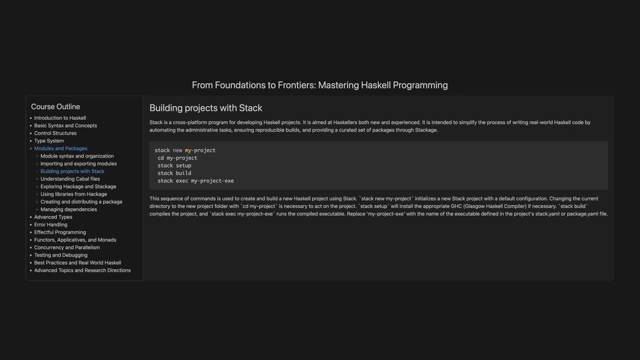 Only nub and sort are available from datalist in this scope: Building projects. Building projects are a set of modules. Each module is a set of modules. Each module is a set of modules. The humbled module島 İnsbagai is designed to build projects with Stack. 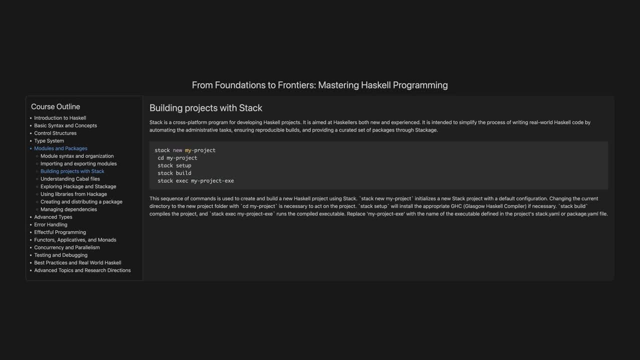 Stack is a cross-platform programme for developing Haskell projects. They are purposes of. Haskell is both new and experienced. The project is intended to simplify the process of writing real-world Haskell code by automating the administrative tasks, ensuring reproducible builds and providing a curated set of packages. 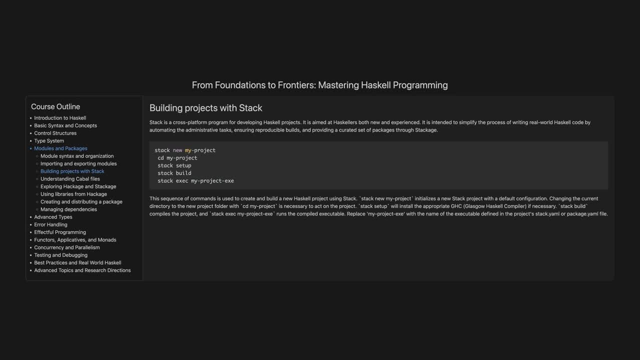 through Stack Edge To resolve the execution of the package. the human code is generated from Haskel modules 5.. with a default configuration, Changing the current directory to the new project folder with cd myproject is necessary to act on the project. 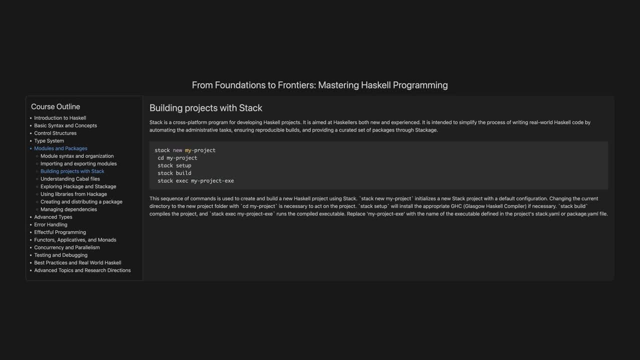 Stack setup will install the appropriate GHC Glasgow Haskell compiler if necessary. Stack build compiles the project and stack exec. myprojectexe runs the compiled executable. Replace myprojectexe with the name of the executable defined in the project: stackyaml or packageyaml file. 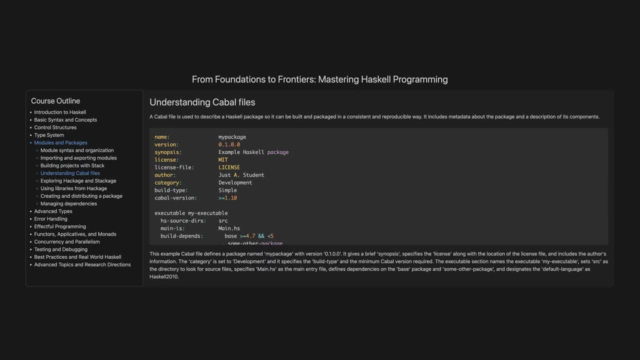 Understanding cabal files. A cabal file is used to describe a Haskell package so it can be built and packaged in a consistent and reproducible way. It includes metadata about the package and a description of its components. This example cabal file defines a package named mypackage. 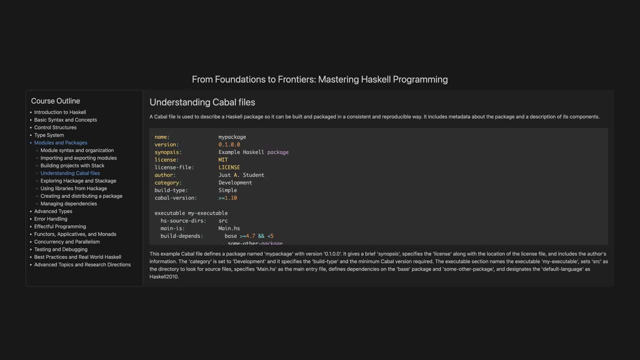 with version 0.1.0.0.0.. It gives a brief synopsis, specifies the license, along with the location of the license file, and includes the author's information. The category is set to development and it specifies the build type. 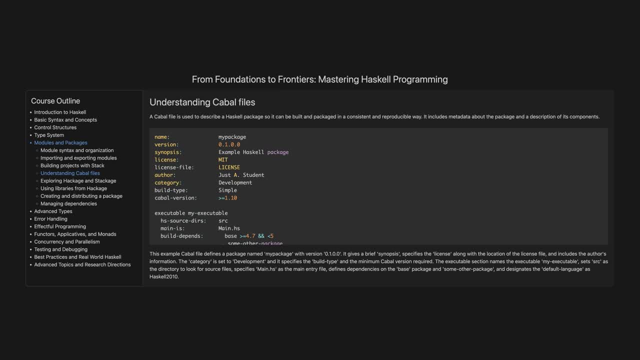 and the minimum cabal version required. The executable section names the executable myexecutable. sets src as the directory to look for source files. specifies mainhs as the main entry file. defines dependencies on the base package and some other package and designates the default language as Haskell 2010.. 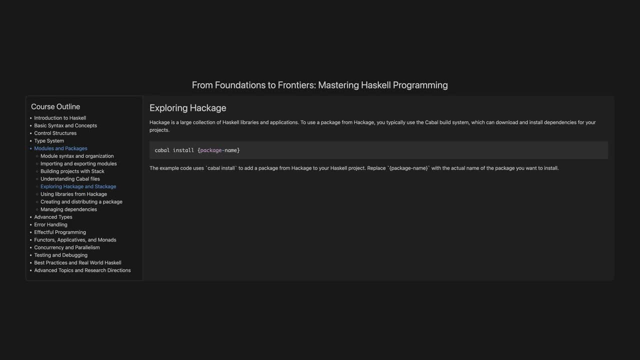 Exploring hackage and stackage Is a large collection of Haskell libraries and applications. To use a package from hackage, you typically use the cabal build system, which can download and install dependencies for your projects. The example code uses cabal install. 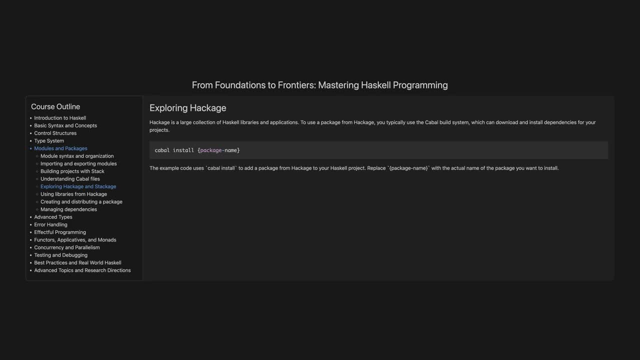 to add a package from hackage to your Haskell project. Replace package name with the actual name of the package you want to install Using libraries from Hack Edge. In Haskell, hackage is the primary package repository where libraries are shared. To use a library from Hack Edge. 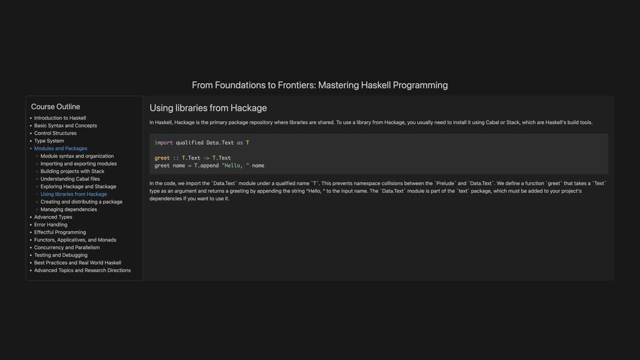 you usually need to install it using cabal or stack, which are Haskell's build tools. In the code we import the data text module under a qualified name T. This prevents namespace collisions between the prelude and datatxt. We define a function: greet. 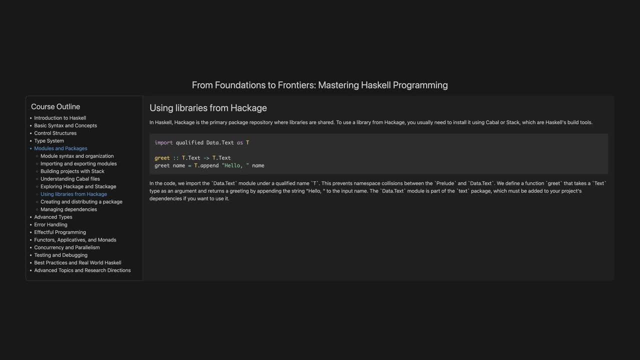 that takes a text type as an argument and returns a greeting by appending the string hello to the input name. The data text module is part of the text package, which must be added to your project's dependencies if you want to use it. Creating and distributing a package. 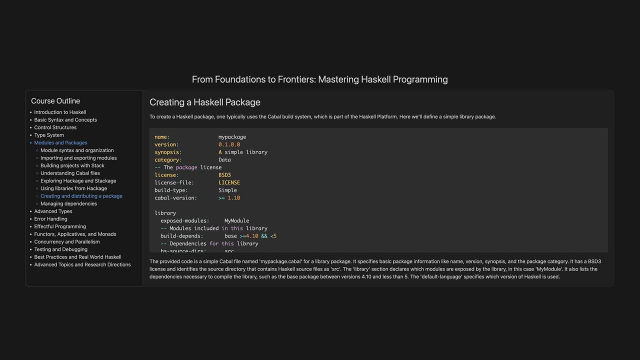 To create a Haskell package, one typically uses the cabal build system, which is part of the Haskell platform. Here we'll define a simple library package. The provided code is a simple cabal file named mypackagecable for a library package. 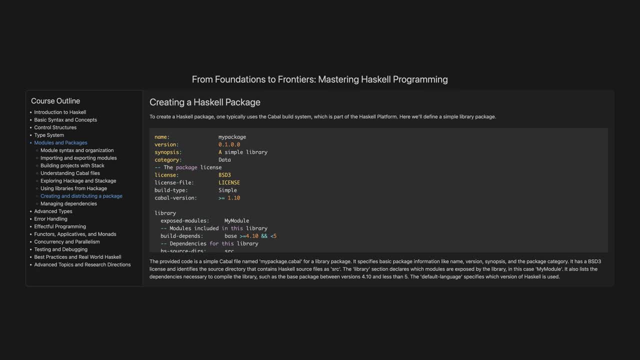 It specifies basic package information like name, version, synopsis and the package. It has a BSD3 license and identifies the source directory that contains Haskell source files as srar. The library section declares which modules are exposed by the library, in this case my module. 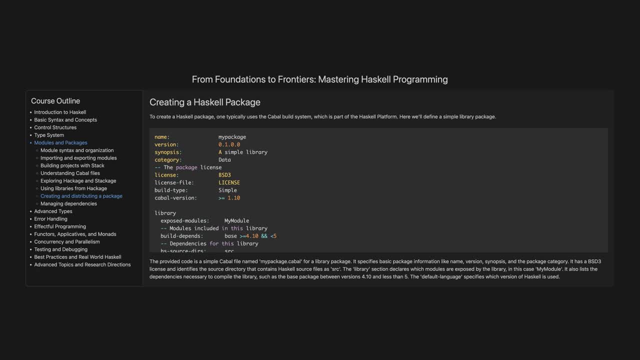 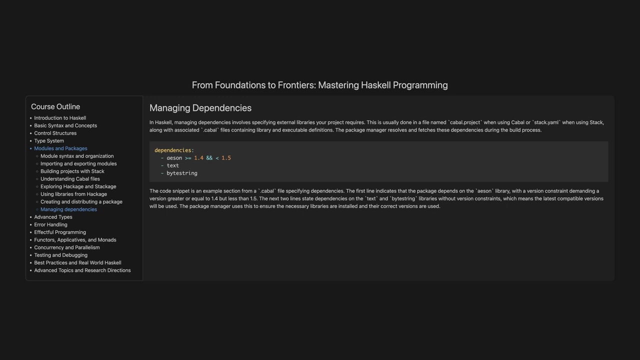 It also lists the dependencies necessary to compile the library, such as the base package. between versions 4.10 and less than five. The default language specifies which version of Haskell is used. Managing dependencies In Haskell managing dependencies involves specifying external libraries your project requires. 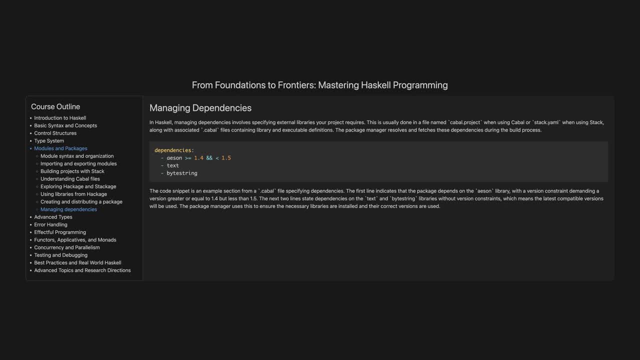 This is usually done in a file named cabalproject when using cabal or stackyaml. when using stack, along with associated cabal files containing library and executable definitions, The package manager resolves and fetches these dependencies during the build process. The code snippet is an example section. 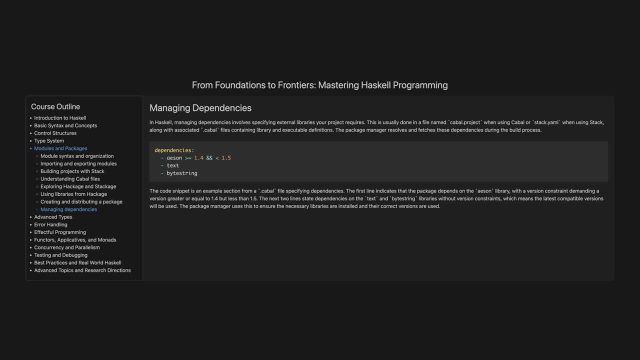 from a cabal file specifying dependencies. The package manager resolves and fetches these dependencies during the build process. The code snippet is an example section from a cabal file specifying dependencies. The first line indicates that the package depends on the ASIN library.